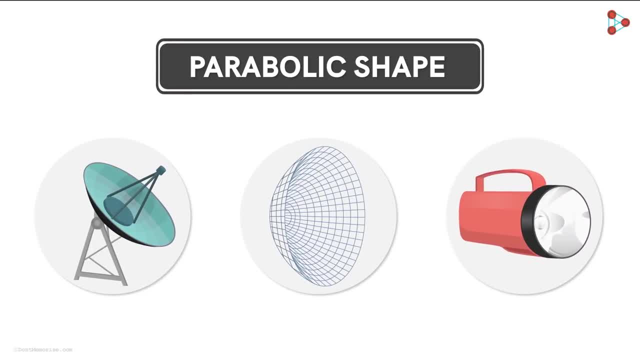 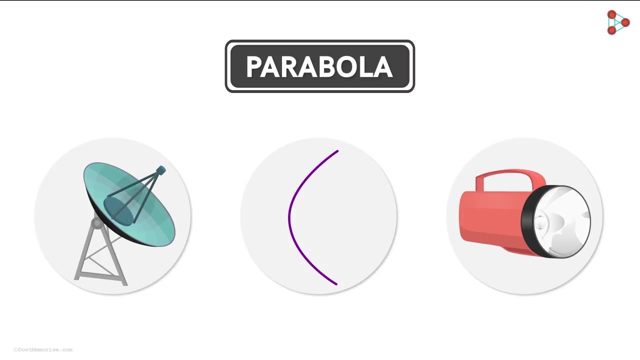 One of them is the mirror used in a flashlight. That's right, It's also made up of this type of a curve. Let's consider just one of all these curves. Such a curve is called parabola. In this video, we will understand what exactly a parabola is. 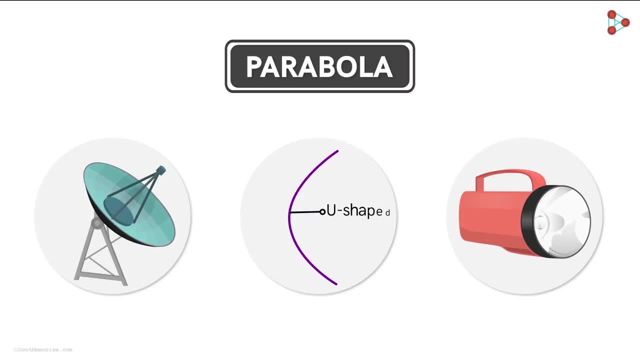 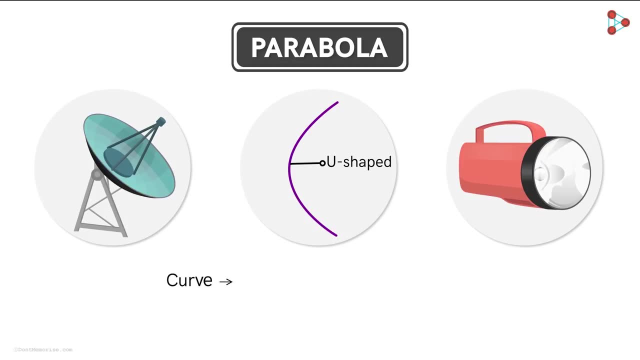 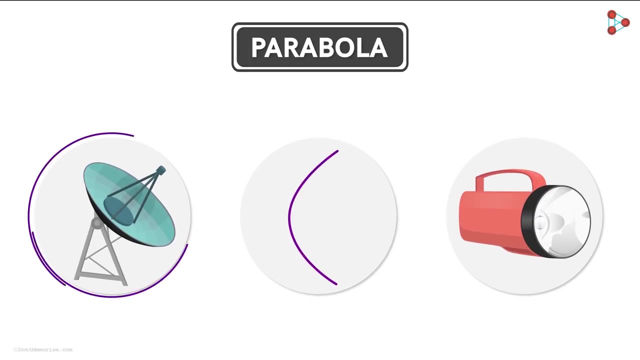 We can see that a parabola looks like a U-shaped curve, But every U-shaped curve is not a parabola. A parabolic curve has a specific property that makes it a parabola. Let's begin with understanding why the dish satellite, or the mirror in the torch, is parabolic in shape. 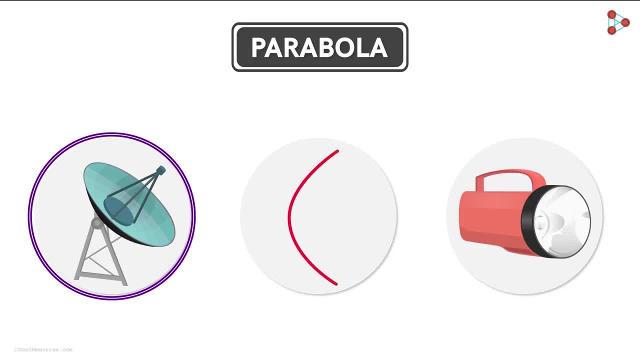 In the case of the dish satellite, due to the parabolic shape, all the incoming signals falling on the dish are reflected towards a single point. This is where the receiver is placed. So the parabolic shape helps in concentrating all the incoming signals at a single point. 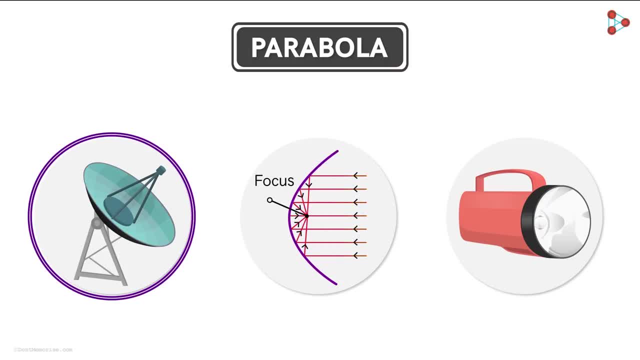 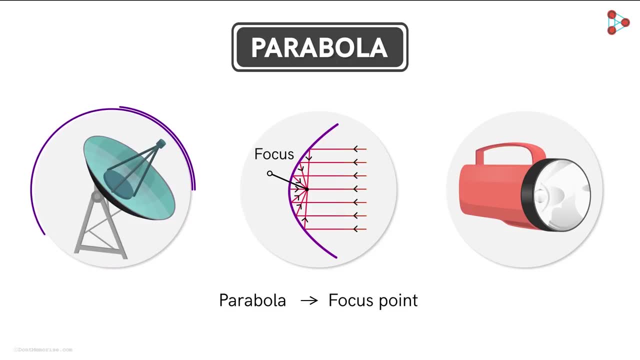 Such a point for parabola is called its focus, And every parabola has a focus point, And this is what makes a parabola so useful. For example, in the case of a torch, a bulb is placed at the focus of the parabolic mirror. 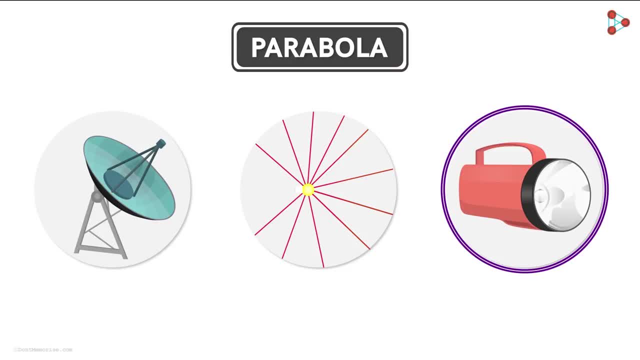 We know, the light emitted by the bulb spreads in all directions, But due to the parabolic mirror, the light emitted in this direction is reflected in the forward direction, like this. So we see that a parabola is a U-shaped curve, Related to which there is a special point called its focus. 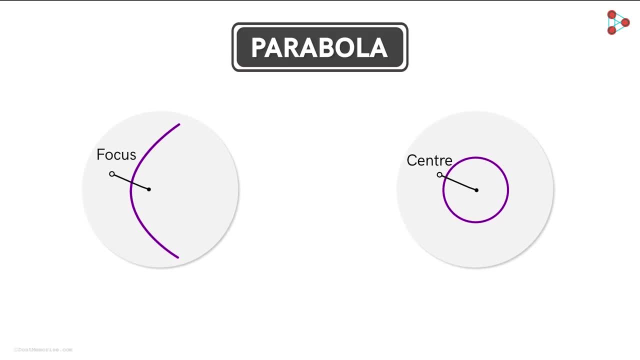 A focus point of a parabola is similar to the center point of a circle, And so, as in the case of a circle, a parabola is actually defined using its focus point. Let us see how. Let's take a point on a plane and name it as point F. 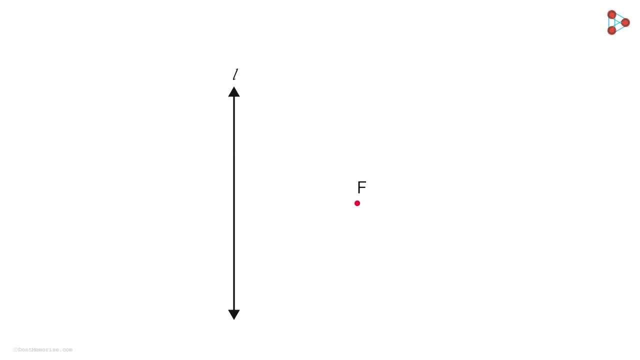 Also, let's take a straight line and name it L. Now please listen carefully to what I'm going to say. next, We will now consider points which are at an equal distance from point F and the line L. Are there any such points on this plane? 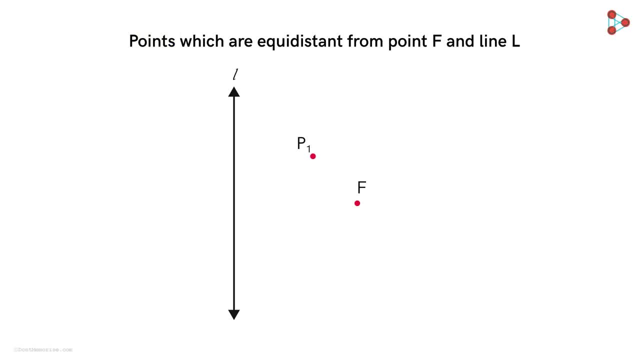 Yes, Consider this point P1.. It will be at an equal distance from the point F and the line L. Consider another such point, P2.. Its distance from point F will also be equal to its distance from the line L, Another obvious point. 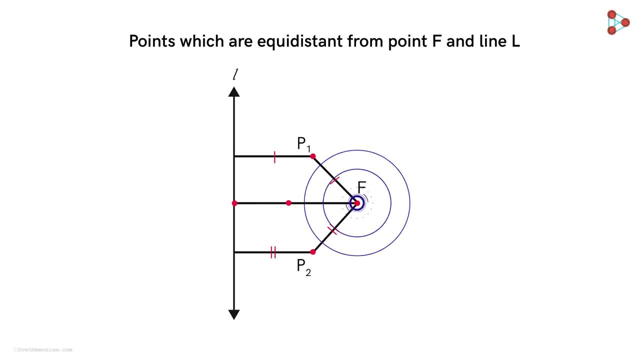 It is the midpoint of the perpendicular segment connecting point F to the line L. All such points that satisfy this condition will lie on this curve, And such a curve is called a parabola. So how can we define a parabola? 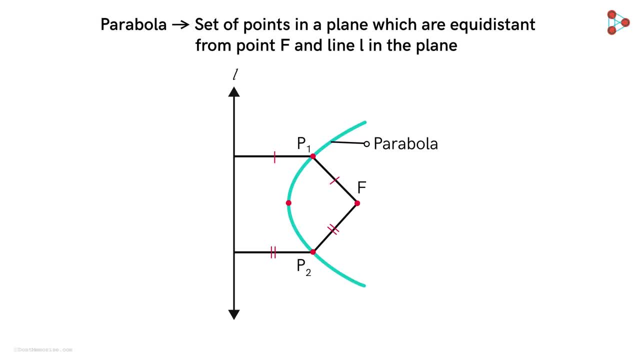 We see that a parabola is the set of all points in a plane that are equidistant from a fixed point F and a fixed line L. They are given special names. The point F is called the focus point, The focus of the parabola, and line L is called its directrix. 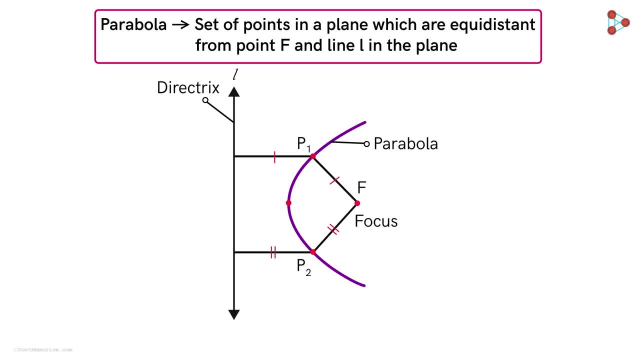 Notice that the shape and the position of the parabola will depend on the position of point F and line L. That is, depending on the point we take as our focus and the line which we take as the directrix, we will get different parabolas. 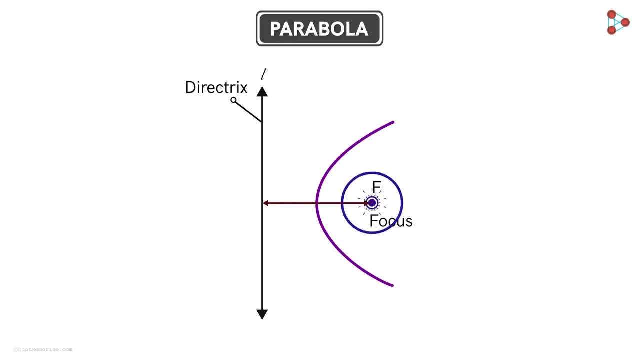 Let's say, for example, we increase the distance between the focus and the directrix here. So let's take this point as the focus and this line as the directrix Corresponding to this focus and this directrix. this will be our parabola. 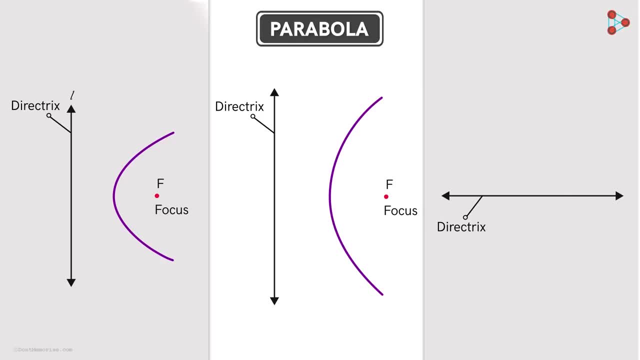 Now say, we take this horizontal line as our directrix and this point as our focus, So what will the parabola look like here? This will be the parabola here. So we see that depending on the focus and the directrix, we get different parabolas. 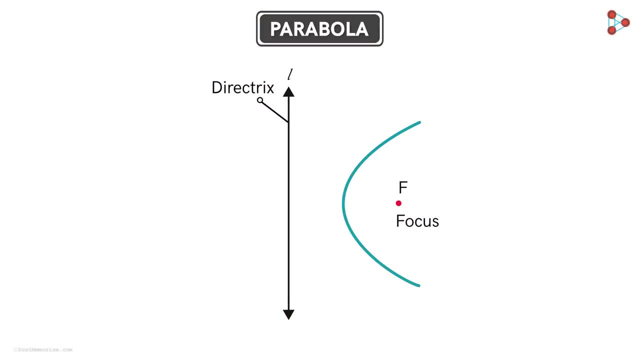 Now consider one last thing. In this parabola, let's draw a line that's passing through the focus and is perpendicular to the directrix. Notice that the part of the parabola above the line is the mirror image of its part below this line. 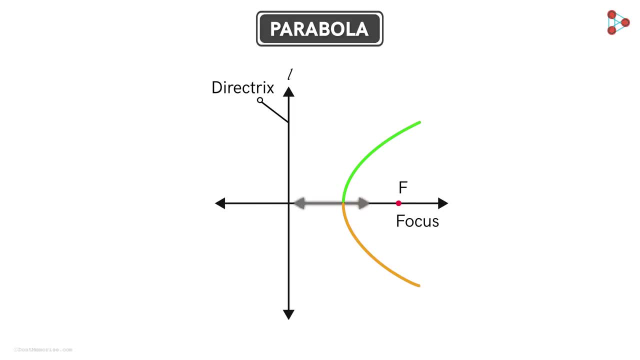 That is, the parabola is symmetric about this line. This line for a parabola is called as its axis, And the point where the parabola intersects the axis is called its vertex. Note that the distance of the vertex from the directrix is the same as its distance from the focus. 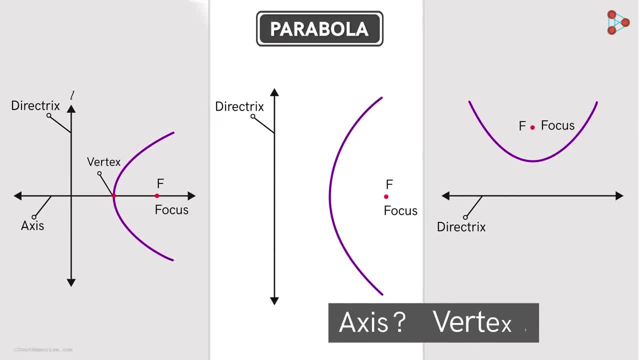 Okay, now can you tell me what will be the axis and the vertex of these two parabolas? For this parabola, this line will be its axis and this point will be its vertex. Similarly, for this parabola, this will be its axis and this will be its vertex.